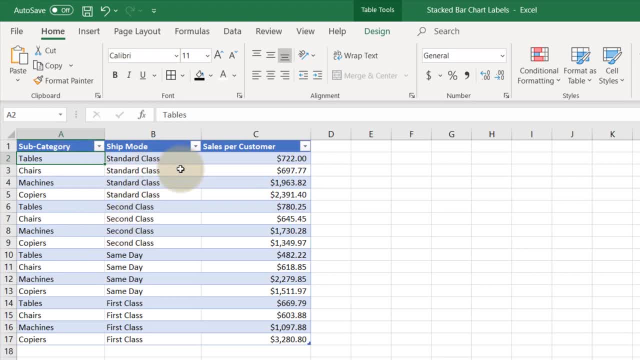 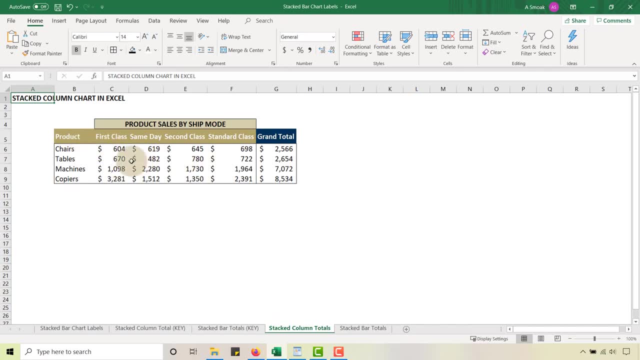 data looks a little bit more database friendly here. You got your subcategory, your ship mode, sales per customer. If we look at what I've got here, all I did was pivot that data to turn it into this. This isn't a pivot chart. I removed kind of the underpinnings there for the pivot. 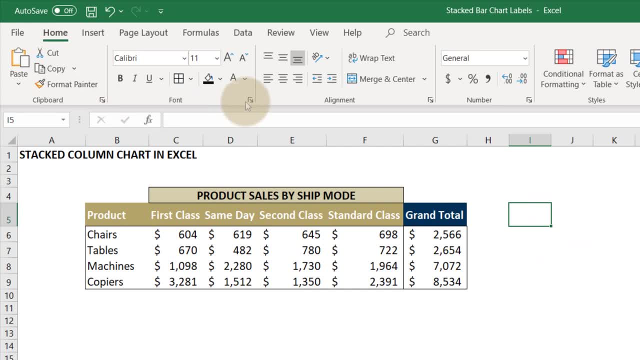 chart. I'm not going to show you how to make a pivot chart. That's not what this video is about. We're going to get right into creating the chart here in Excel. So let's highlight all of these, the products, and let's highlight the ship mode as well, And I'm not including the grand total here. 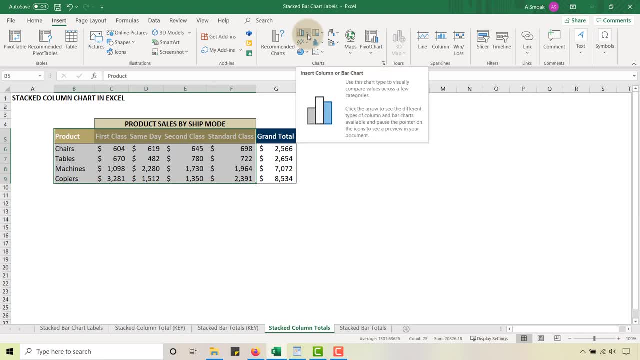 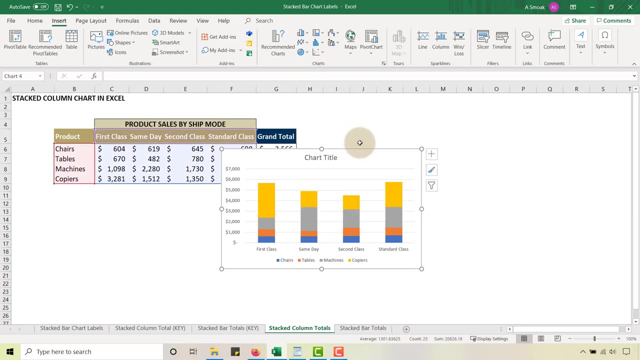 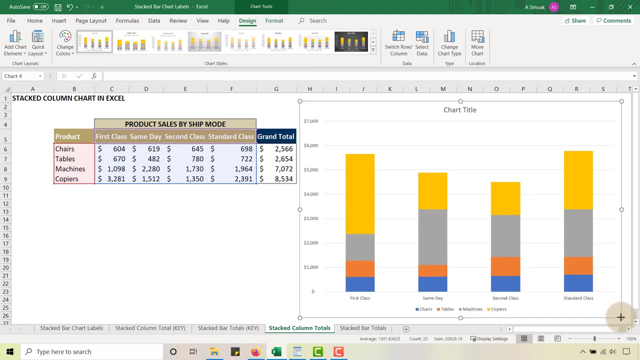 And then, once we have those highlighted, we can come up here and we can insert a 2D stacked column right here. All right, So we have something like this, And then I'm just going to go ahead and make this a little bigger so we can see that And we can do a little bit of formatting. 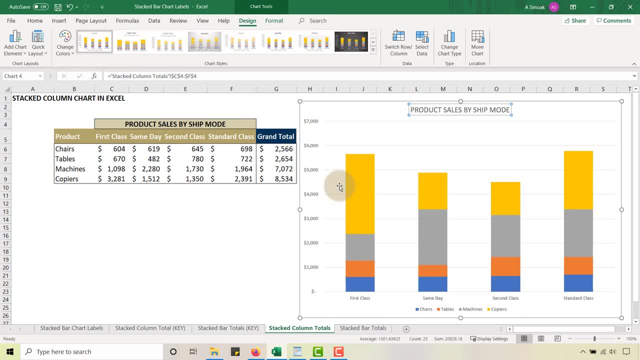 here I can say equal to this right there. And if you'll notice, I have see how we have the first class same day, second class, standard class. Those are the columns up top here What I want. I want my first column here. 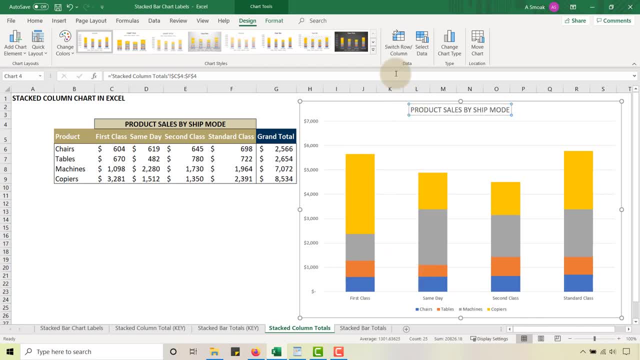 To be on the axis. So what I like to do- I mean, you could do it either way, But what I like to do is I like to switch the row and column So you'll notice my chairs, tables, machines and copiers are. 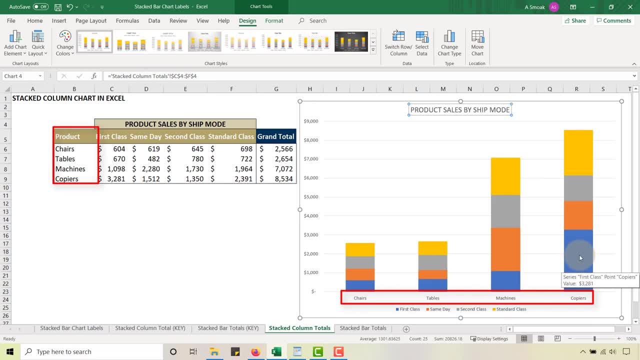 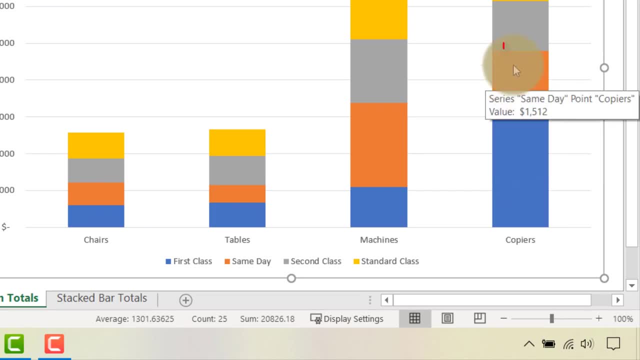 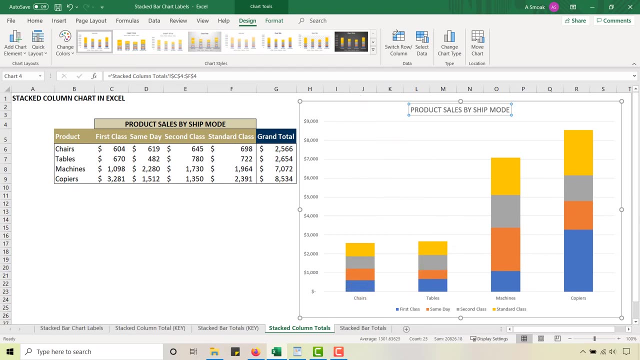 here on the axis And then on these different cuts, right, I should have right copiers. So this is all copiers. Sorry, First class, same day, basically my ship mode. So once I'm in this, in this format right here, what we can do here, we'll just do a little bit of formatting here. 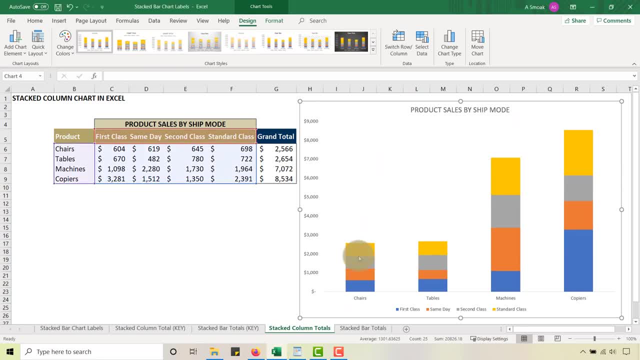 I'm going to delete this right here And then you can go to add labels and bring in all of your labels. Do that fairly quickly, Right? And so all of those were correspond to, um, to the different values here in these subsequent, uh, subsequent- columns, right? So what I want to do is get all. 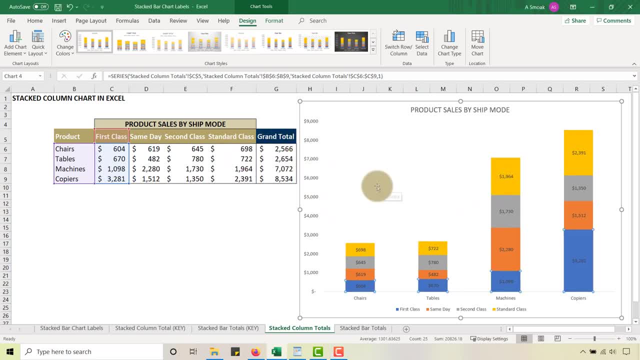 the grand total stacked on top here. It's a little hack, So in order to do that, let's select uh. right, We select the chart and then we can expect- uh, we can expect that we're going to get all the. 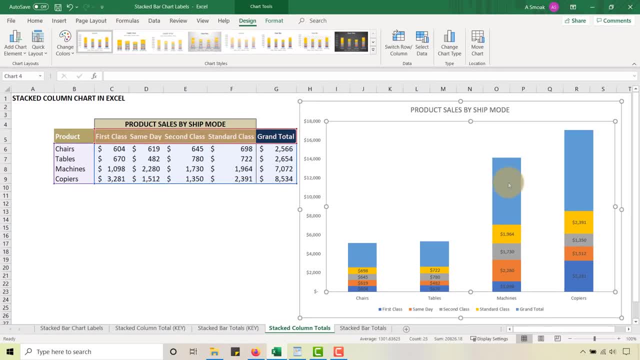 and the chart here to include the grand total, And you'll notice we have this big chunk here that corresponds to our grand total. So if I select copiers here, you'll see the value of 85,, uh, 34,, which corresponds to copiers, And we can actually turn, uh, we can add data labels there. 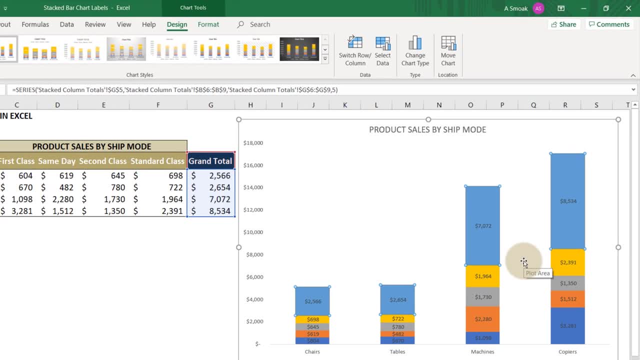 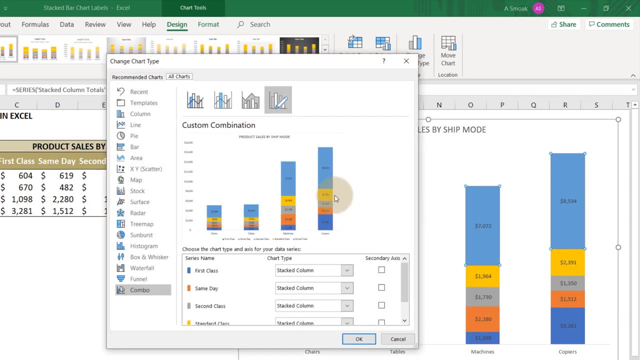 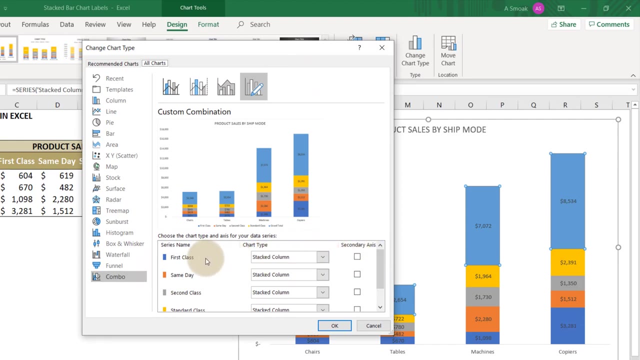 So you can see that that is the grand, uh, grand total. And so what we want to do now, let's go in here, Let's um, let's change the series chart type, And this will pop up right, We're in a combo chart- and write all of these um the ship modes. 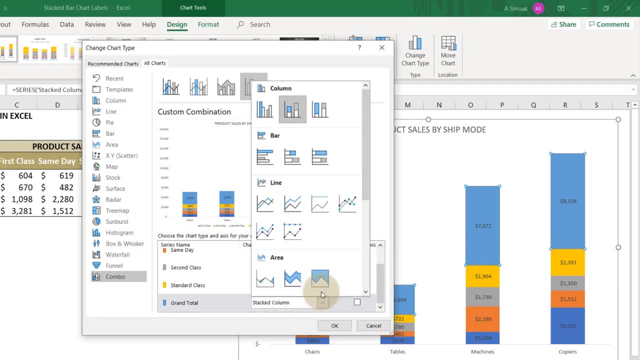 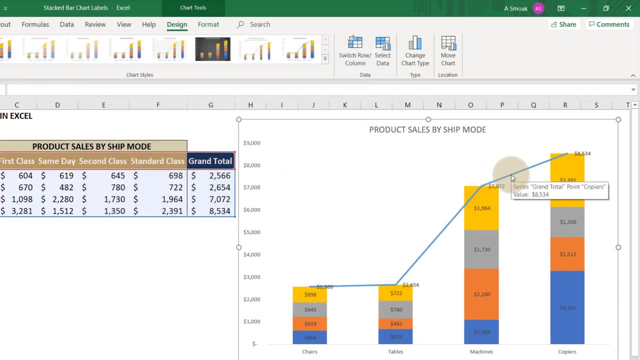 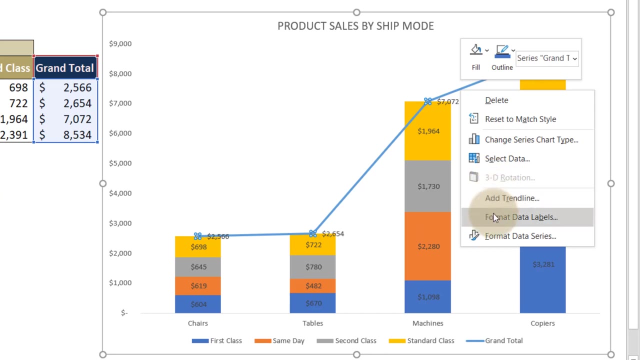 We want to keep a stacked column, but on the grand total, I want to change this over to a line. right, Say okay, And we end up with something like this: And then I'm going to go in here and make sure that you select the whole line. I'm going to right click here and let's go ahead. 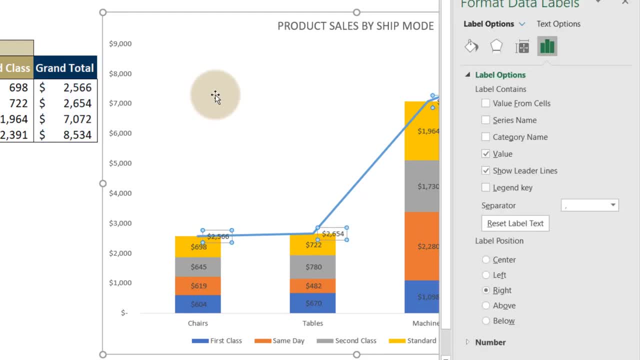 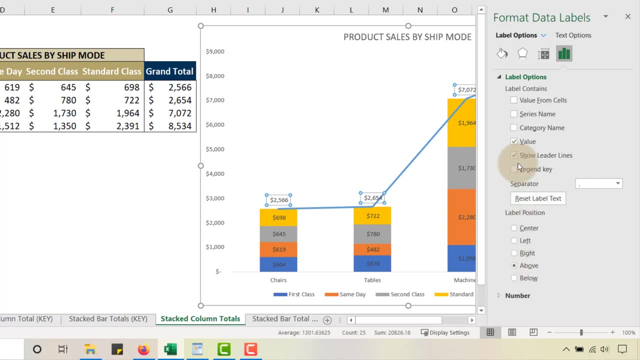 and format the data labels And those should show up at some point And I want to make sure that those are above and you'll see that they move there And I can leave that. uh, leave that alone for now, And then we can get out of here. I'm going to come back and make sure I'm selecting the the line. 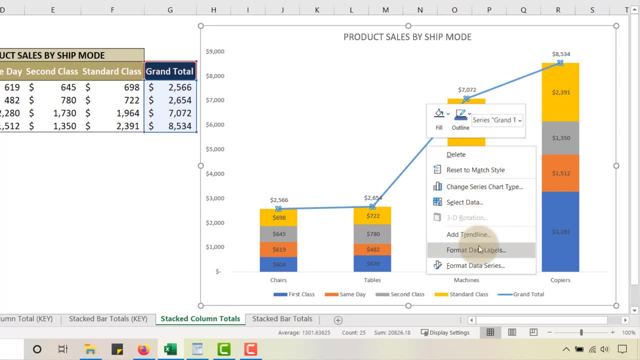 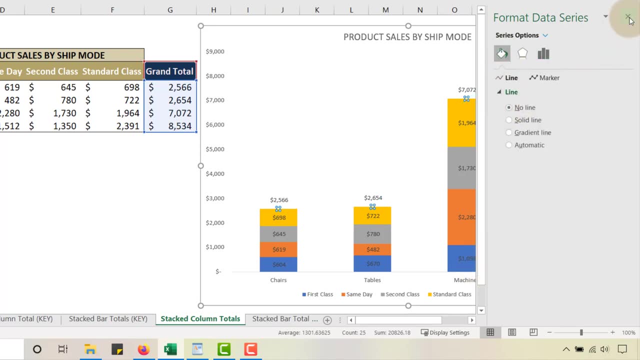 You'll see all the points here, And then I'm going to uh uh, format the data series And if I come over here I want to say no line, right, And that gets rid of our line. And so now all we have to do, I can select these: 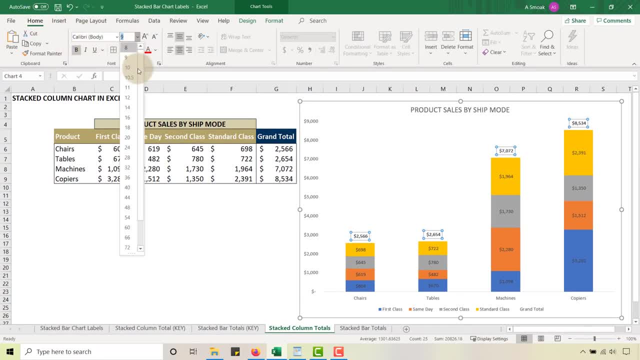 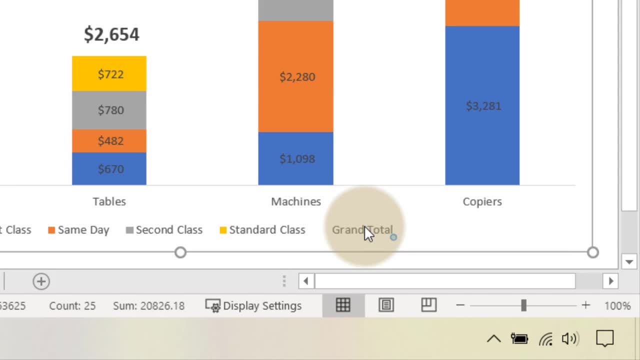 and just format this as normal. I can make that bold, I can make this a bigger if I want to make that stand out And you'll notice, we have the grand total down here. We don't want that grand total to show up, So I'm going to select it and hit delete And there you go, We have our stacked. 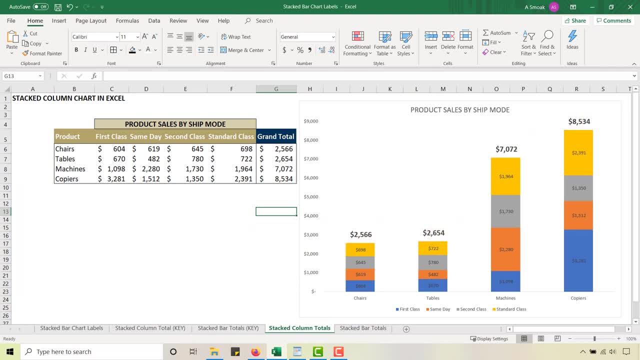 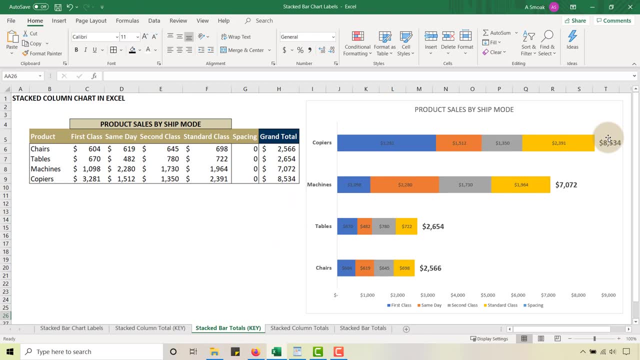 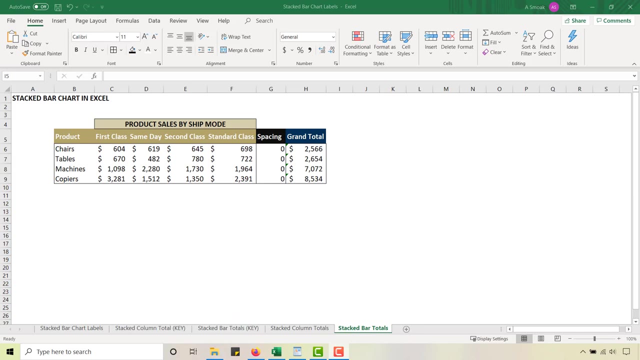 column with the totals on top. So that's part one. Now stick around, I'm going to show you the stacked bar totals. Let me show you this guy right here, how we add those totals to the stacked bar totals. So stick around, Okay. So the stack bar chart in Excel adding totals: this one, this is: 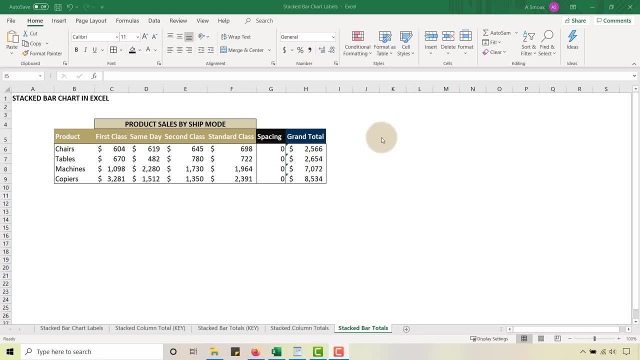 the one you want to stick around for. This one's a little bit trickier, a little bit more hackier. You don't see too many solutions for this on the internet, So so this is the one you want to watch, So let's go ahead and highlight. And well, first thing, you'll notice, I have this new column. 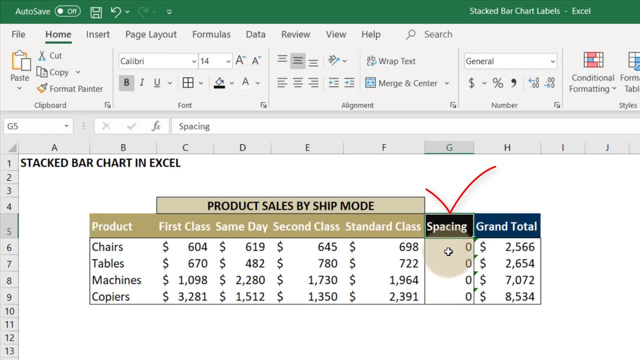 called spacing, right? So you'll want to put this column in here. I call it spacing And you want to have a? you know we'll. we'll start with a value of zero. I'm going to change this, so you. 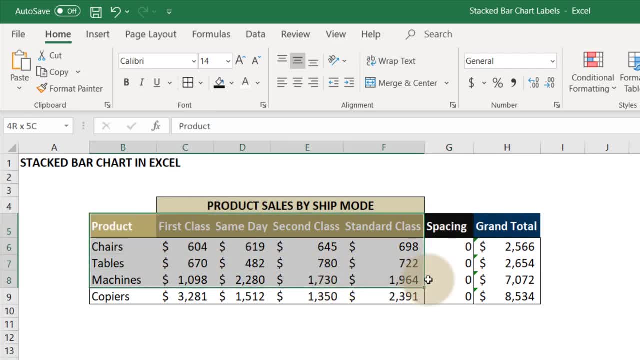 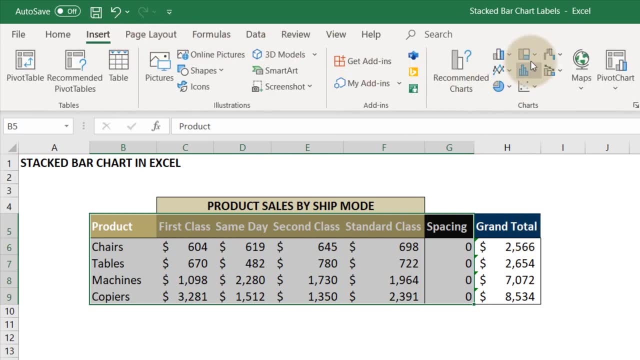 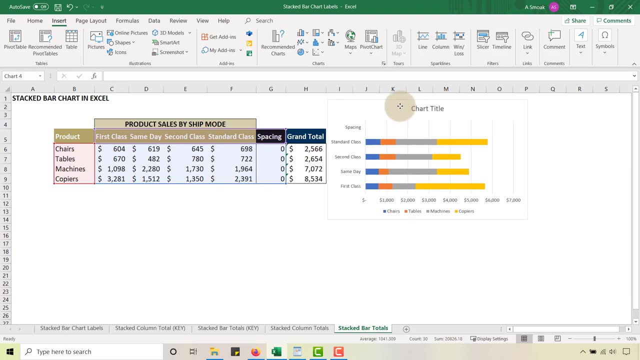 can see, but we'll start with this. So let's highlight all of this, not including the grand total, And then we're going to go up here to insert And we go back over here and we want our 2D bar And we end up with something like this: Let's go ahead and expand this out. 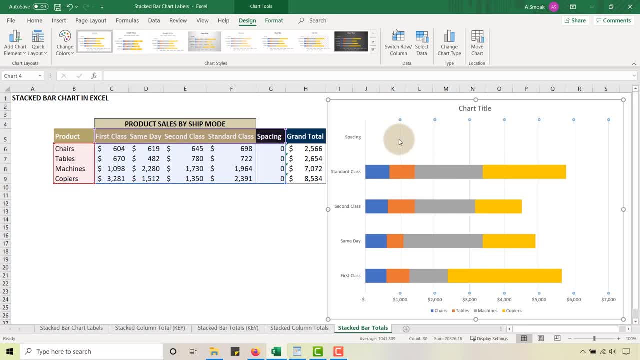 So it's easier to see, right, And we're going to do our little formatting, get rid of that, do our chart title Here we go, All right And you'll notice. right, So spacing is here. Basically, again, I want my products to be on the axis so I can switch the row and column And you'll notice. 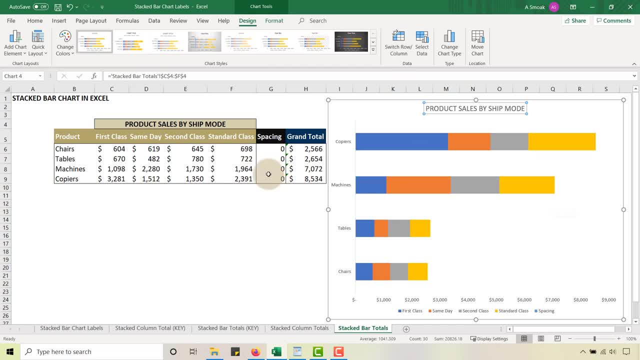 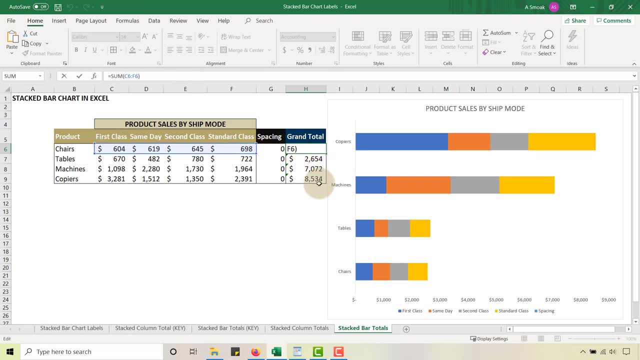 that spacing disappears because it has a value of zero, right, And we want to make sure that our grand total does not include the spacing value, because we're going to change it. It's only a summing up these values, So all right. So what do we do with, with that, that spacing value? So, 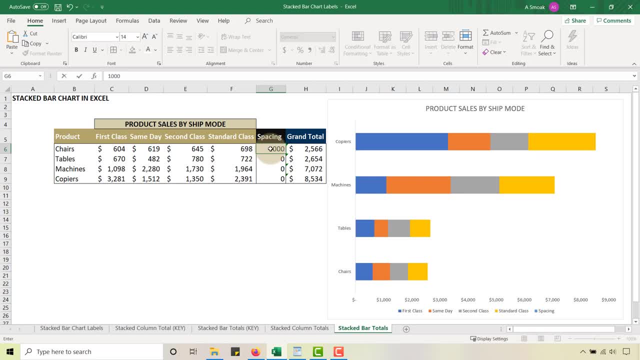 right now, just temporarily, I'm going to put a value of a thousand in here, just to get something to show up right, And so you'll see, right, I could copy this down, but I don't want to screw up my formatting. So you'll see, I've added this spacing value here. Let's go ahead and turn all. 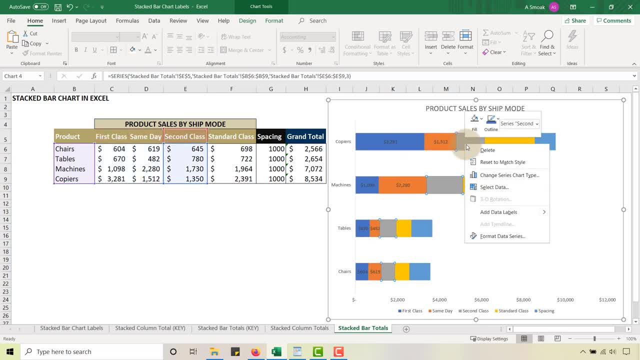 these on, just so you can get a feel for, um, what these correspond to. I'm going to go add all those data labels and I'm going to add the data labels for the spacing. It has a value of a thousand right here, And so what I'm going to do, I'm going to go in here, I'm. 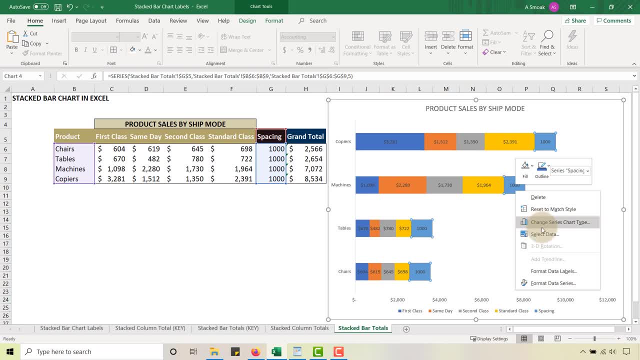 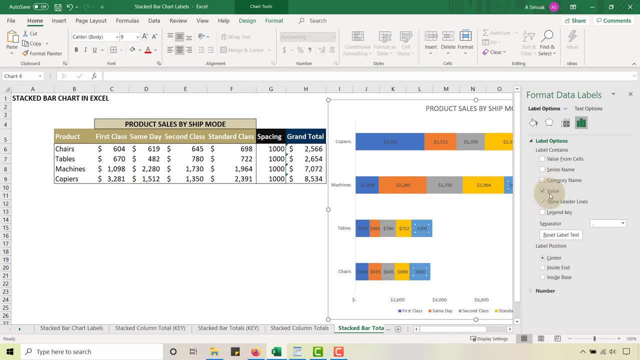 going to right click And then I want to um format the data labels and you'll see it has a value here And what I want? I want the value from cells, not the value, the value from cells. So I'm. 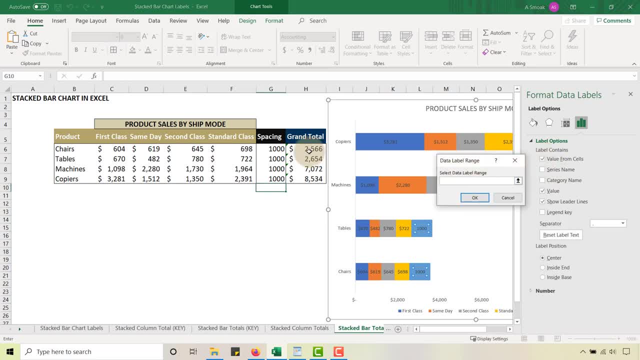 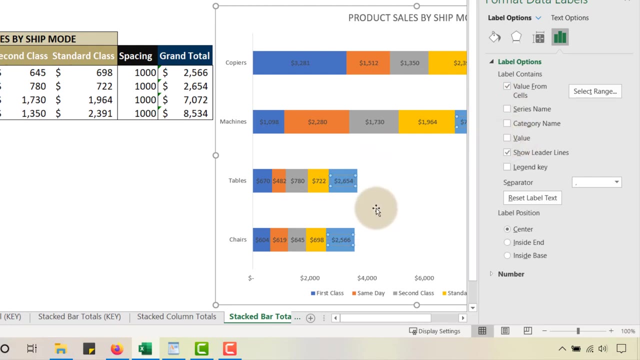 going to select value from cells. Uh, it's going to ask me for a data label range. I'm going to go without the headers, say okay. So what that does. you'll see that it's trying to put in two values here. It's putting in the value and the value from cells. If I uncheck value, you'll see. 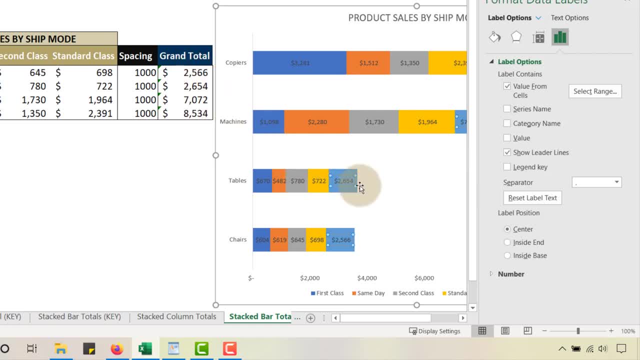 that my thousand now is replaced by the grand total. So that's what that value from cells does. And let's go ahead and format the spacing data labels. Let's move this position here, uh, to inside base. So we're going to, we're going to move that to inside base. 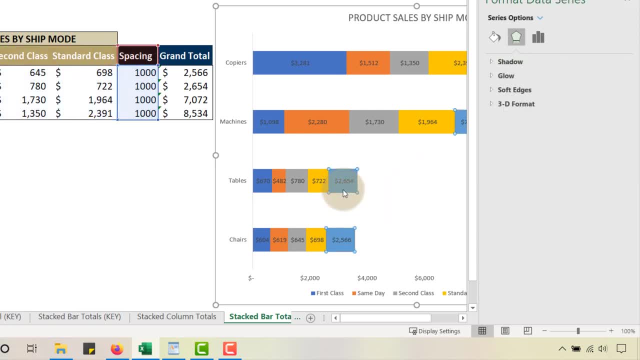 And then I'm going to select. I'm just going to go back in here and select the uh, the series here And we want to change the fill to no fill, Right, So now we just have our value, just kind of. 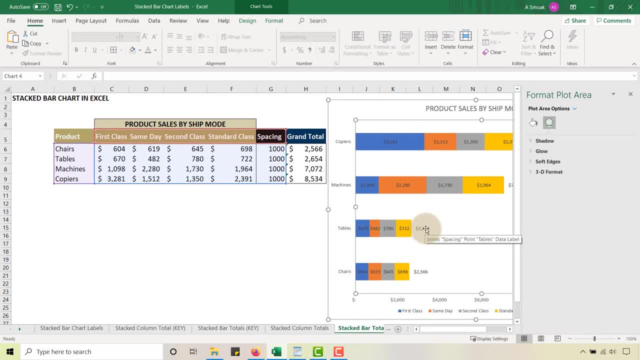 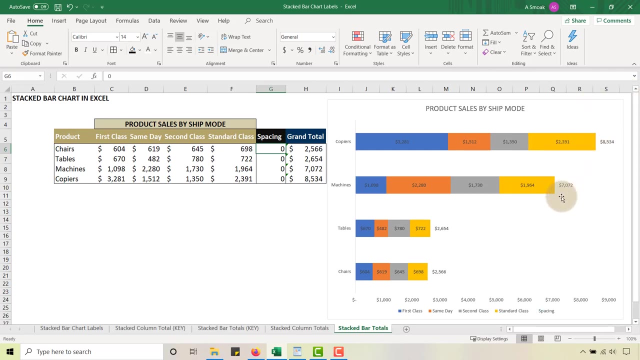 floating out here, right, Changing it to inside base keeps it, keeps it right there, And so what I can also do, I can go back and change these to zero, just in case, Right? So if I change those to zero, um, you'll see that. oops, get rid of that. You'll see that my values are still here. 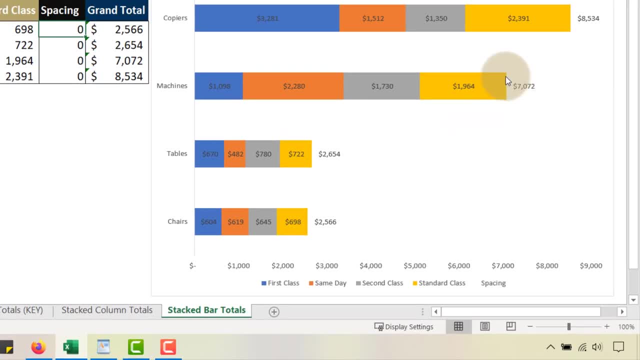 Right, So a little hacky way of doing it. Basically, there's a zero value here, but we're showing the grand total instead of the zero. I mean, that's, that's the uh, the trick right there. And of course, obviously we can do some, uh, some minor formatting, just like we did before. 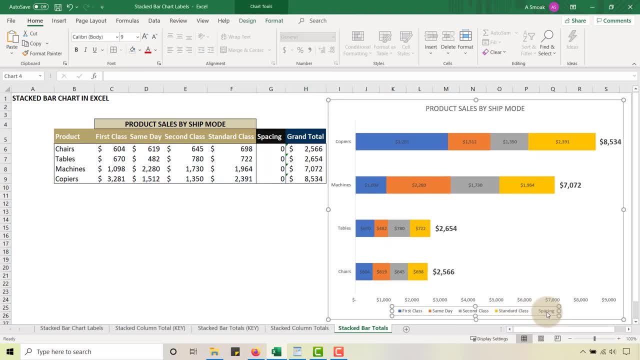 make that stand out, make that pop. I want to get rid of my spacing value. We don't need to see that. And then you know, you know you can do something like this. You can uh format the legend If you. 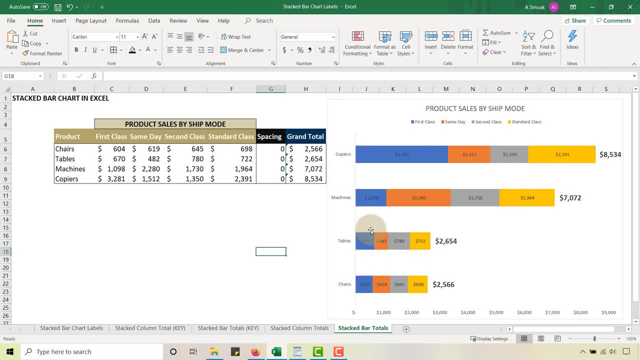 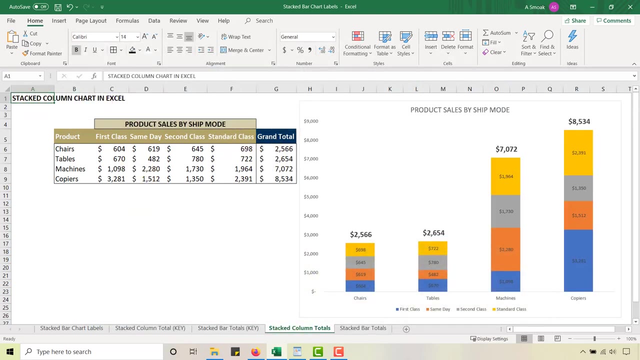 want to go around, you can. you can do that, Just showing you a little extra tip. but here you go. This, this is how you add totals to your stack uh bar chart in Excel and your stacked column chart in Excel. So hopefully this has been helpful. as always, This is Anthony smoke. 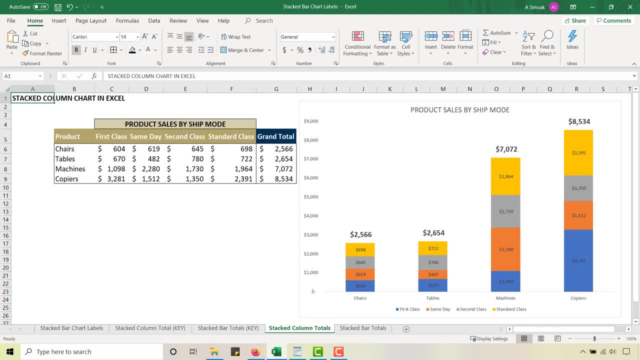 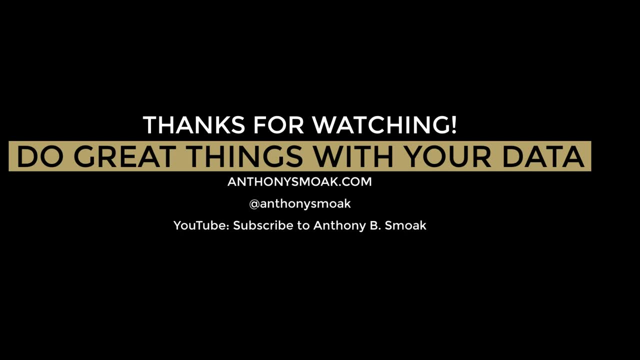 Get out there and do some great things with your data. Thanks for watching.